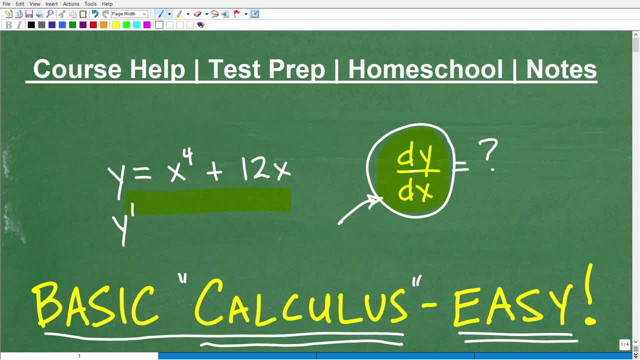 steps to knock out. It's gonna be a pretty short video But before I get going let me go ahead and quickly introduce myself. My name is john. I'm the founder of tablet class math. I'm also a middle and high school math teacher And I'm going to leave a link to my math help program in the description of this video. But basically I have 100 plus different math courses, ranging from pre algebra to pre calculus and everything else in between. So if you're at those levels, which are generally middle school, high school and even college level mathematics, I can 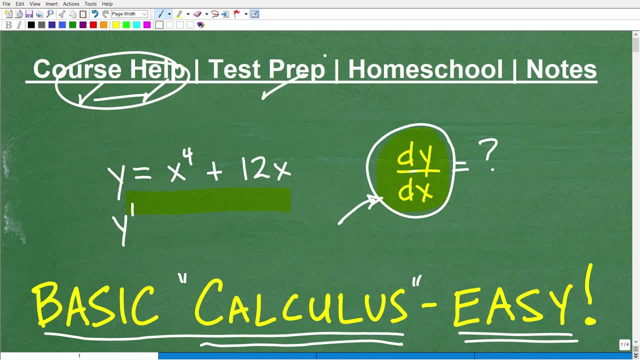 help you out If you are taking a test that has math on it- So, for example, the GED, SAT, ACT, GRE, GMAT, ASVABACUPLACER CLEP exam, maybe a teacher certification exam- you get the idea. if it has math on it, I can help you prepare and pass those exams. If you homeschool, I have a very comprehensive homeschool math curriculum you might be interested in, And if you don't have any math notes, you can use mine. I'm going to leave links to my math notes in the 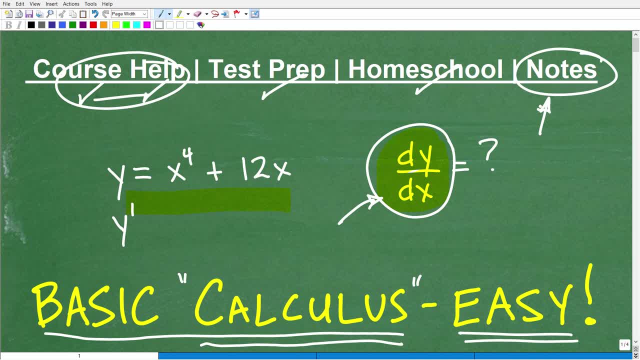 description of this video And I'll see you next time. this video, but you got to start taking notes. no way you could survive in a course like calculus, or any math class at that, without taking excellent notes. so just take great notes, you'll thank me. 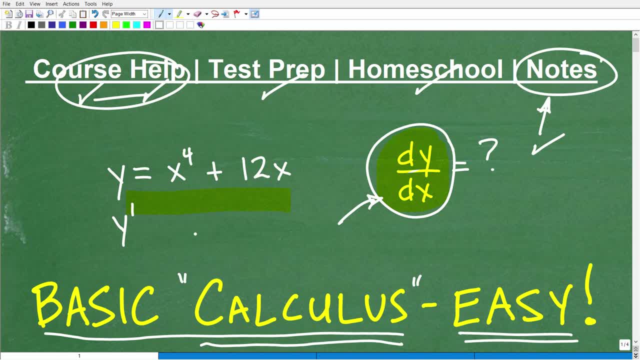 later now let's get into this first derivative business. now. i'm just going to show you how we can calculate or well, actually find the first derivative of this equation right here- that's kind of the idea- and see that the steps are very, very easy in order to do that. but let's just try. 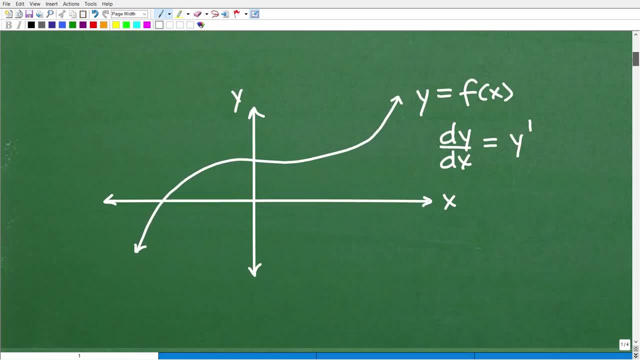 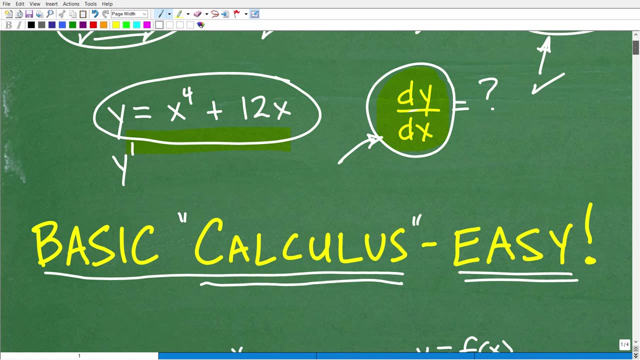 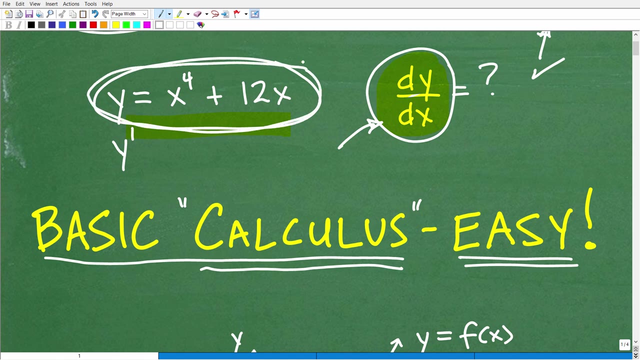 to get a sense of what the first derivative is. now again, i have more videos on this if you really want to get into it, but just a quick review. so we have this equation. this y equals- let me just go back up here: y equals x to the fourth plus 12x. now, with this equation- and by the way, i'm kind of- 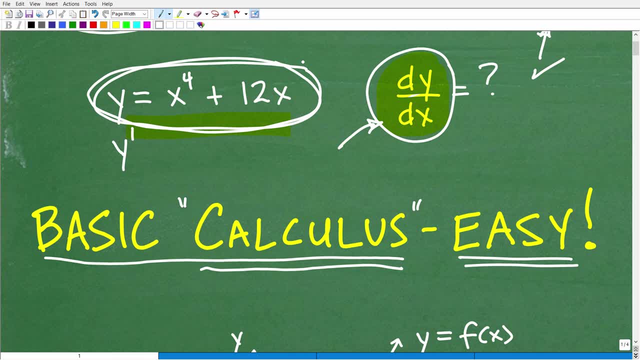 very, very informally talking about the first derivative. so those of you out there that maybe are phd in mathematics and you teach calculus at a college level, obviously you would be teaching, you know, in a more formal sense. i get that. i'm just trying to explain this so that any, uh any- person kind of get a basic. 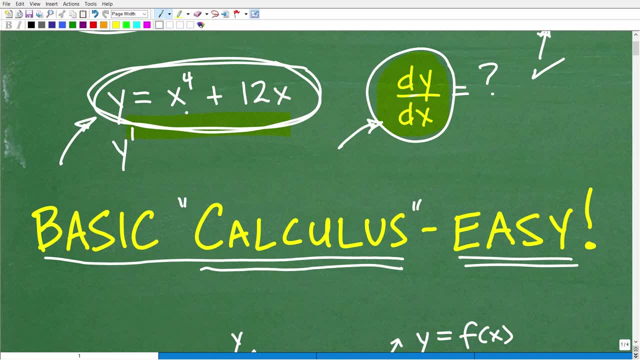 idea. so here we have this equation. now this equation: uh, if i put a little f of x in front of this y, okay, y and f of x are basically the same. so in other words, i could write this: uh, right here, this y equals x to the fourth plus 12x, as f of x is equal to x to the fourth plus 12x. so this is a. 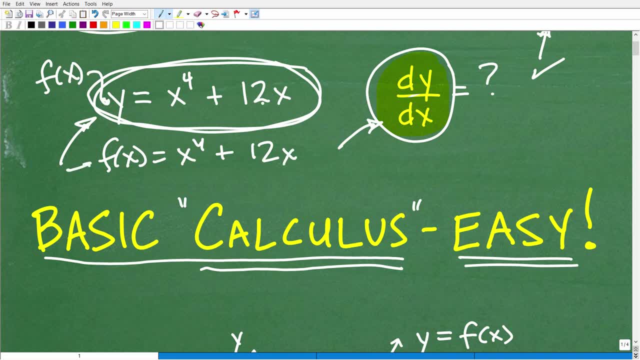 function. this is an equation, but basically you can kind of see that the first derivative of this equation here, which is the first derivative, is the будемic scale dimension, because actually the first derivative is the bottom part of the song. okay, and the first one is the prove, Oh. 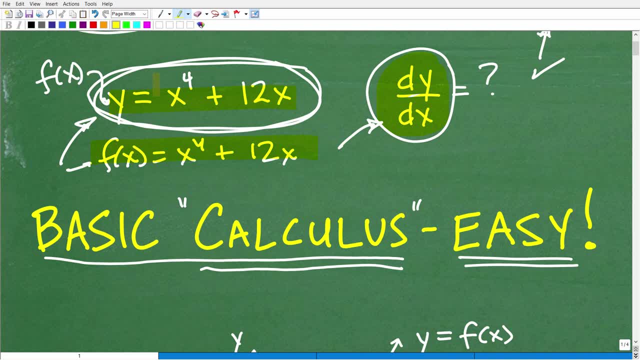 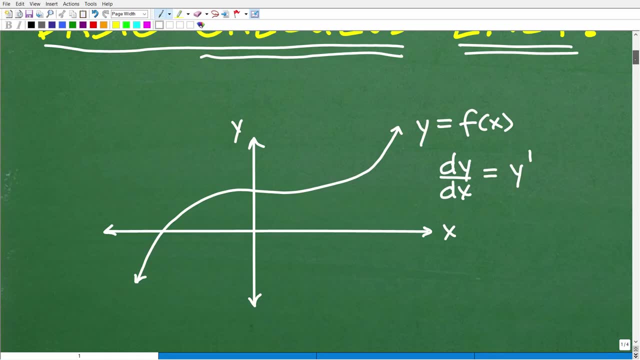 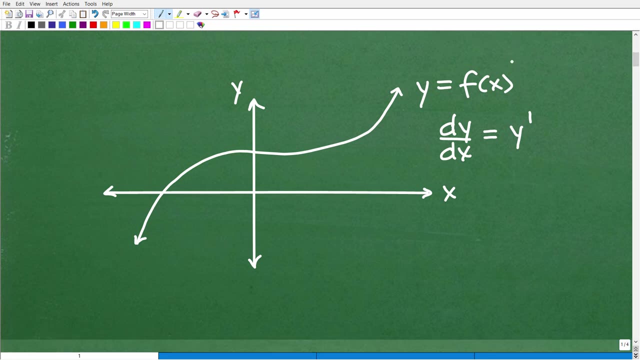 to the equal, and we really don't even have an entire song right here. so we have a sufficient process to come to the fundamental term, and when we come to f of x- ysics, you actually have to make this a setup function. so if i were to start with f of x, 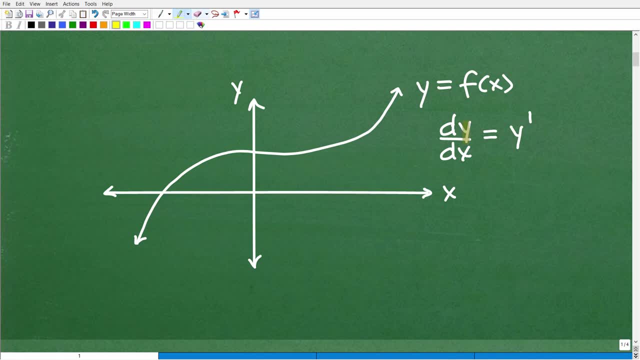 on this LOVE in. and then we'd add this letter f of x to this 결 other equation and it's going to result in a problem. this dy dx- it is the same way to express- that is y prime. so we're talking about a function or this little y notation. this is y prime. but basically we're talking about something called. 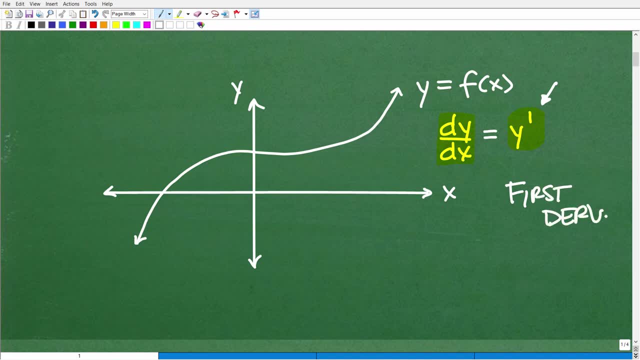 the first derivative in calculus. okay, so you can find the first derivative, the second derivative, even the third derivative, and those have all implications, especially for things like if you're taking a physics, physics course, etc. etc. but we're just talking about the first derivative. so in calculus we have this thing called an integral. okay, now we kind of think of this as 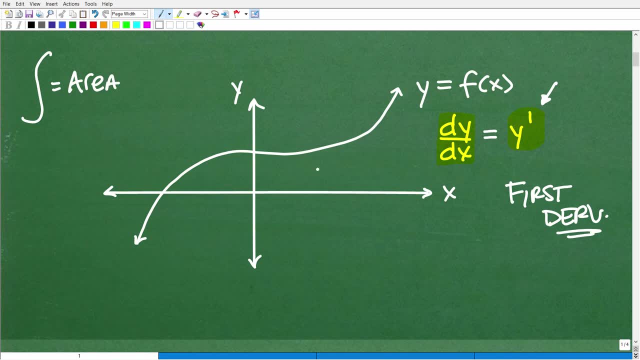 finding the area underneath a curve, like right here we have a curve and if we wanted to find the area underneath it, we would use this integral symbol. okay, again, i have additional videos on this in my playlist, but we're using this symbol. okay, we're talking about this. this is the other half. 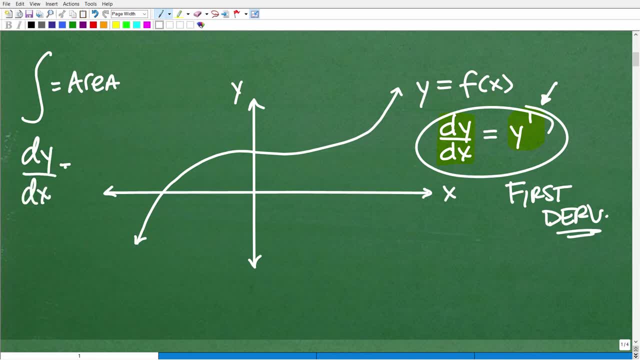 of calculus, this dy, dx, and this is the derivative. okay now, a great way to think about the first derivative is to find the area underneath a curve like right. here we have a, the derivative, and it's precisely what it is: it's an equation for the slope of this curve. okay, so 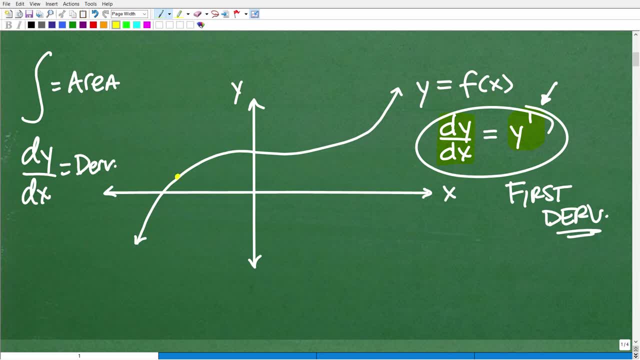 here I have this function, this graph. so, let's say, I wanted to find the slope of the of this function, this graph, at this specific point. okay. so like, hmm, what am I talking about? well, I'm talking about what's the angle right here? okay, what is the angle at this particular point? well, 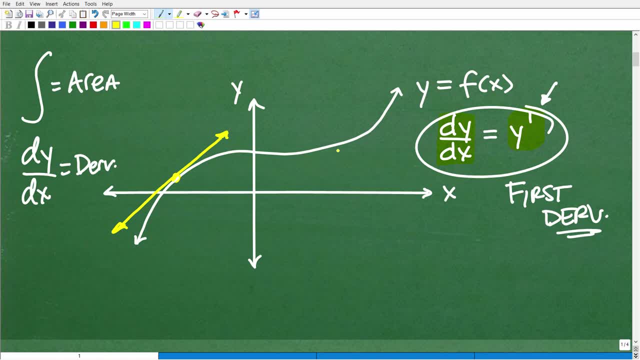 it might be something like that, this line here we call this the tangent line. but let's look over here. what do you think the angle of this function is right here? this graph, well, the slope might be something like this right, and so you could see that this is always changing. I'm going to kind. 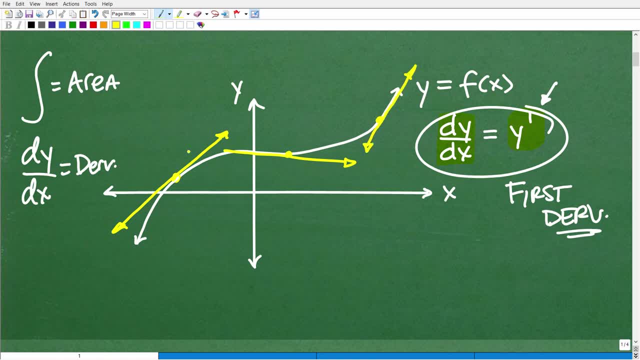 of try to kind of sketch it right here. so the slope is constantly changing along this graph. all right, well, the derivative is the first derivative is basically the equation for the slope. so you effectively what the first derivative can do if I have a function and I go find this first. 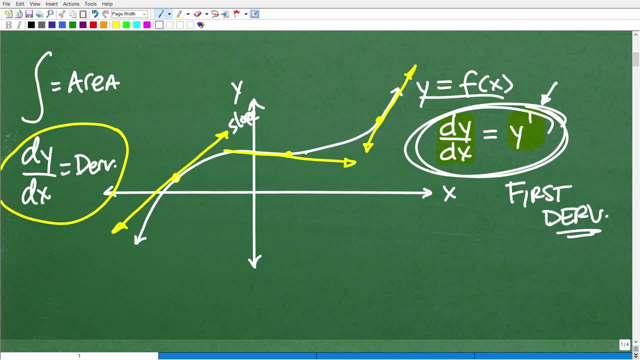 derivative. I can find the slope anywhere along this graph that I want and that has serious implications, very, very powerful. we also call this the rate of change, okay. so why would I call that the rate of change? because you can see this is changing. okay, this is obviously changing again. 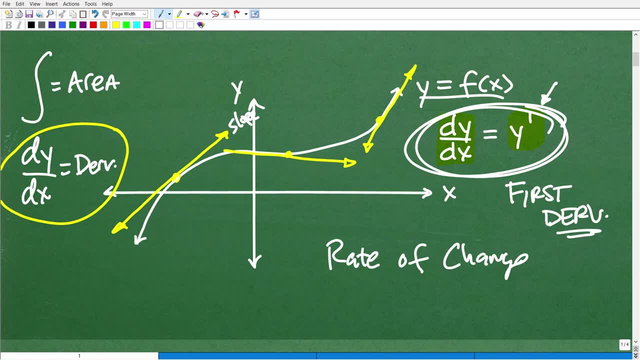 I don't want to get overly technical, but this is what we're trying to do. okay, so we're given some function, okay, so I'm some y equals some equation and has an associated graph, and we're trying to find the first derivative, this thing, which, again, it will give us the slope of anywhere along this graph that we desire to you. 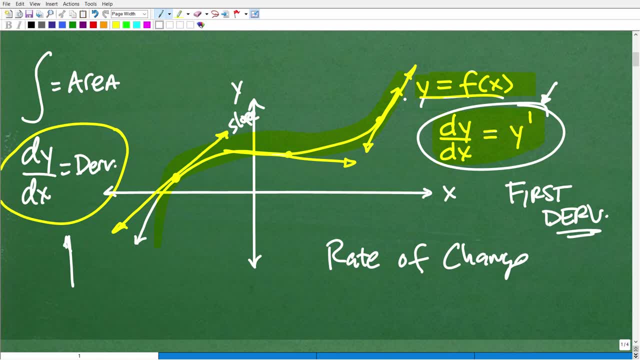 know to explore. okay, so hopefully I did a pretty good job of explaining the first derivative. I mean, this is obviously very, very. you know, I distilled down to the most basic sense, but that's the whole point of this video, so let's get into it. So let's get into the actual application of finding the first derivative of this problem. 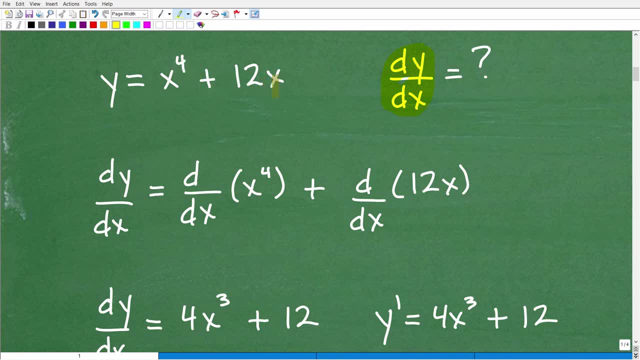 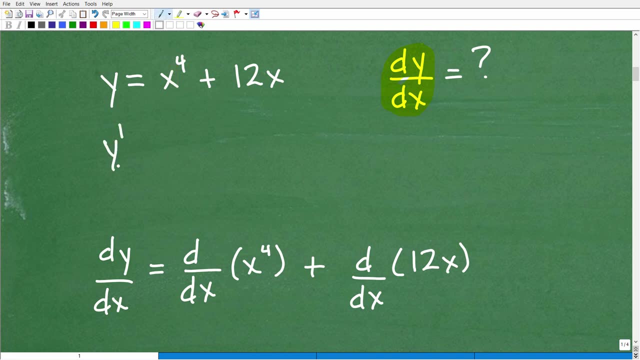 OK, so here we go. Y equals X to the fourth plus 12 X. Now I'm going to show you. I got a lot of crazy notations. All we're going to do Y prime. That's how we say that Y prime is the same as this notation here. 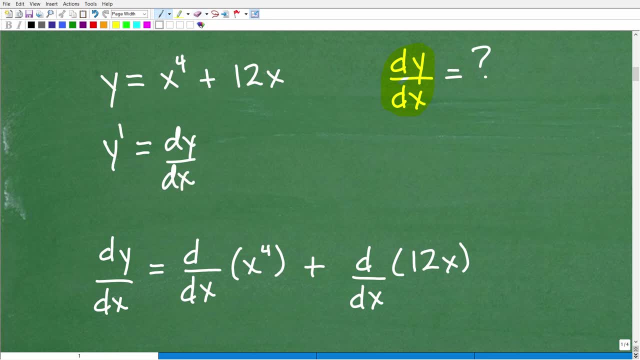 D, Y, D, X. OK, it's the same thing. So all we do- and I'm going to explain this part right here because I'm kind of shown a little more formally- is the following: OK, when you're finding the first derivative, basically in calculus, you learn a bunch of rules. 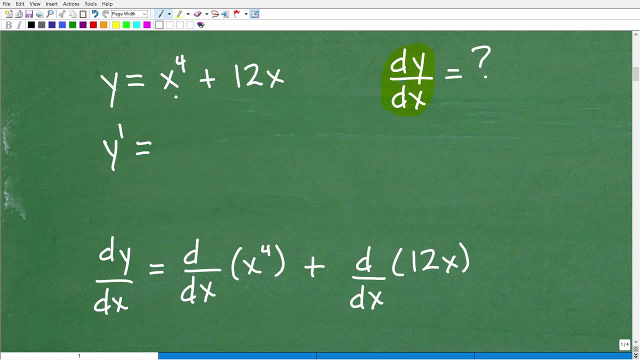 All right, But the rules aren't overly complex, Just rules. So anytime we have like a positive power, OK, that's an integer like- so we can do this. I see this little four right there, And in front of this X is actually a one. 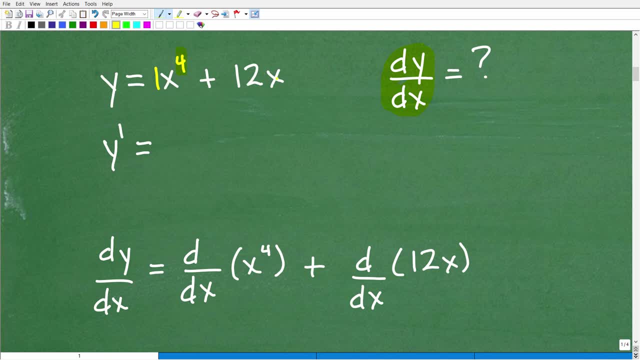 We don't write that, but that's what it is. And then over here I have 12 X. What's the power here? Well, it's to the first power. OK, so just watch this. Here's the rule that we apply. anytime we have a positive integer, like so, we take that four. 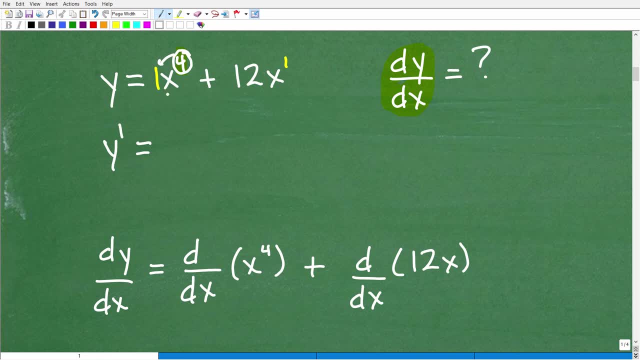 OK, we multiply it by whatever number is in front of the X, or could be any other variable. So four times one is what it is for. OK, then I'm going to write my X. Now you see this four right here. All I'm going to do is subtract one. 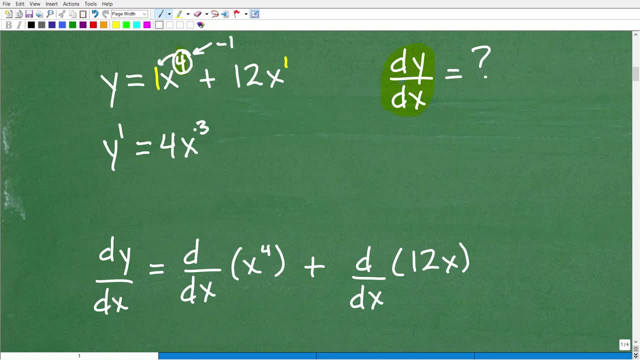 You're always going to subtract one. So four minus one is three, Pretty easy, OK, that's all we do, And then we're going to go on to the next term. OK, so we have 12 X to the first. So one times 12 is what, That's 12.. 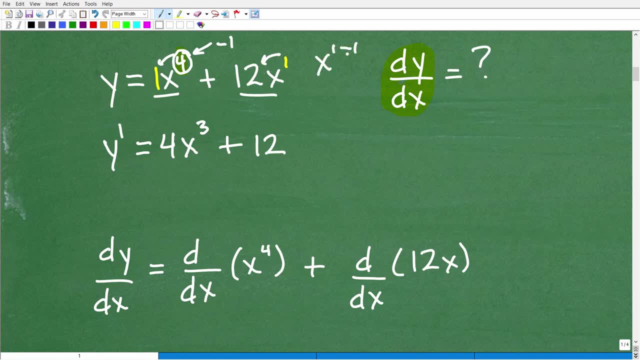 So X, OK, one minus one. I'm going to subtract one again. is what? X to the zero, Anything to zero power is one, So it's just going to be 12.. OK, so this is the answer. Right, Super easy, We are done. 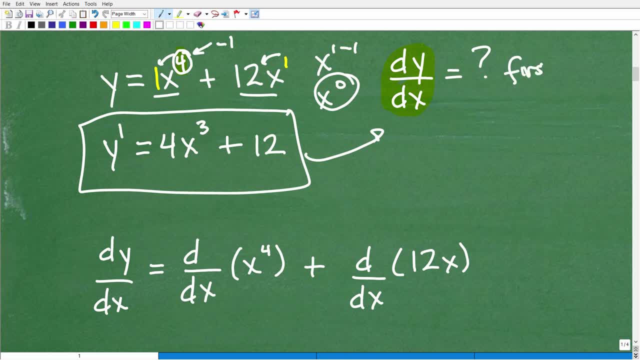 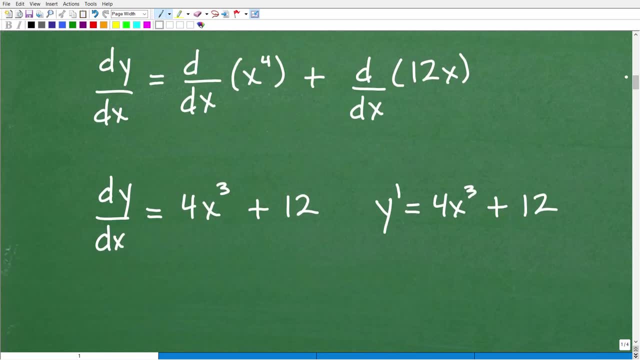 We just found D, Y, D X, which again is The first derivative. All right, So let's go ahead and just look at this a little bit more formally. So when you're looking at this you're like: oh wow, this looks more complicated. 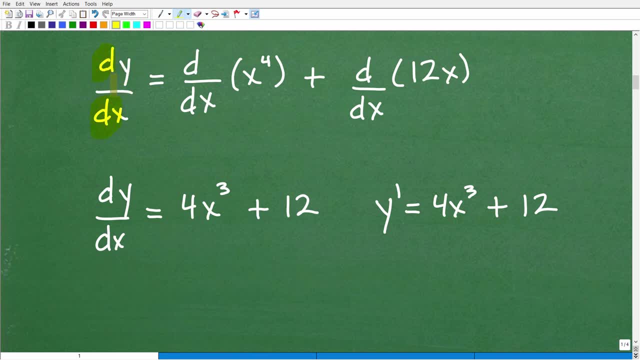 Well, it's not OK. so here I'm going: D Y, D X, Right, And we're going to take the derivative of each one of these things. This is going to be D? X of this first term, And we'll write it the same way this way. 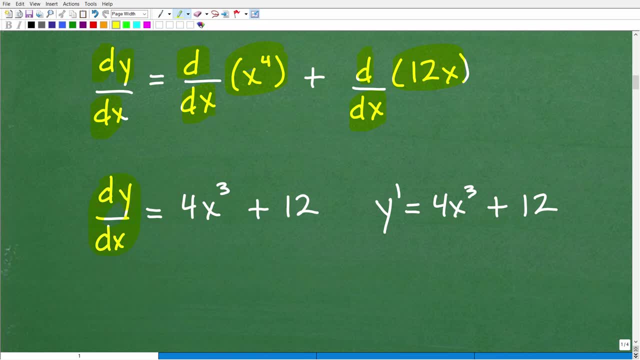 So in more formal calculus symbology we would find the first derivative, which is the same as that Y prime, D, Y, D, X. And here's the answer again, for X cubed plus 12, or Y prime is equal to four X cubed plus 12.. 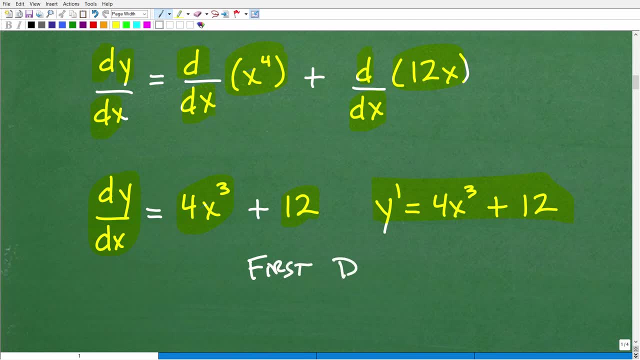 Again, this is the first derivative And you're going to have to find the derivative of their derivatives first, second and sometimes, you know, additional derivatives of all kinds of functions and calculus. But you know, this is not that difficult. I mean literally. we just, you know, went four times. 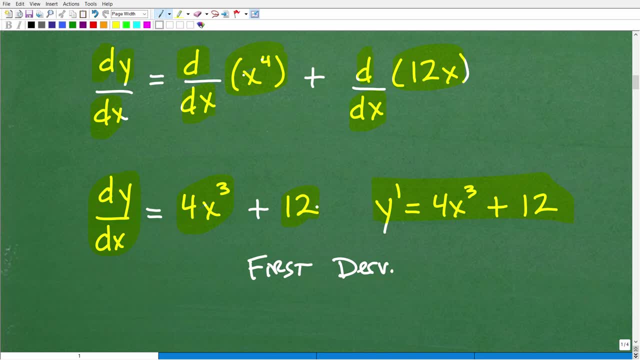 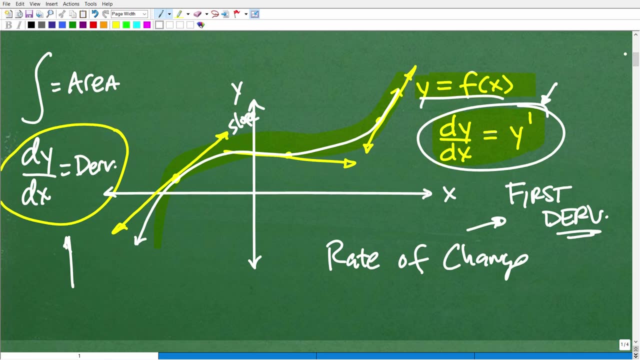 One is four, Four minus one is three, Like one, two, three Right. So calculus is a lot of. it is not that difficult, And of course you have to understand the concepts And it's certainly much more you know, you know involved than what I'm making it out to be. 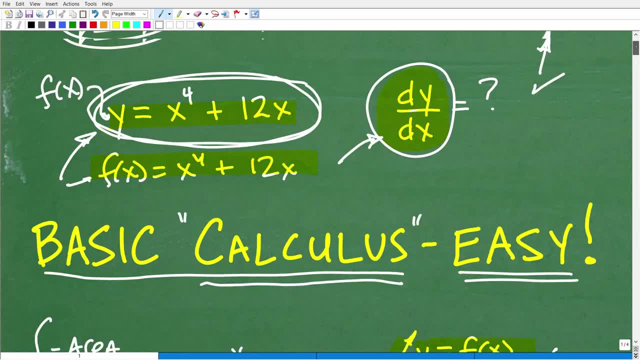 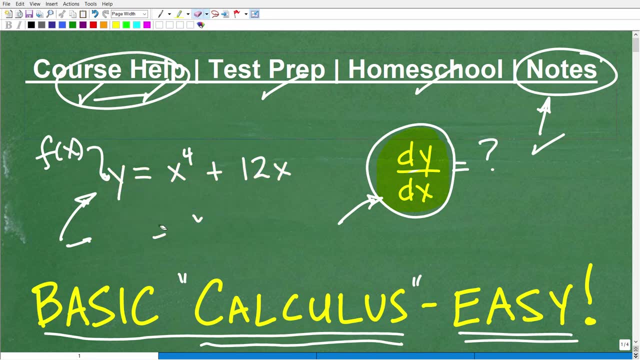 You know it's not going to be like super easy. when you take a calculus course, You're going to definitely be challenged, But don't be intimidated by the concepts. OK, so if you understand this well, you just found the first derivative, first derivative of a function, and you just learned some basic calculus. 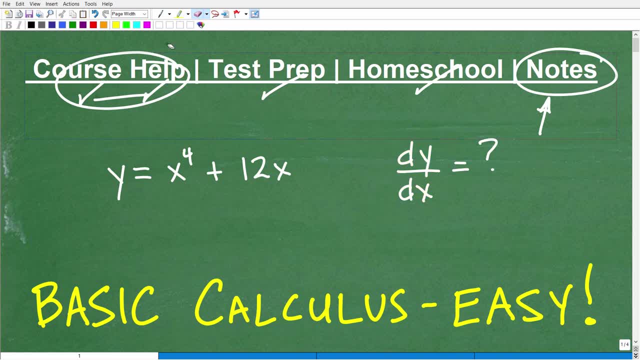 OK, I would certainly encourage you if you're interested, if you're on the fence, you're like: should I take calculus? Should I work towards doing that? I would definitely encourage you to take calculus because it's just will like just show you the power of mathematics. 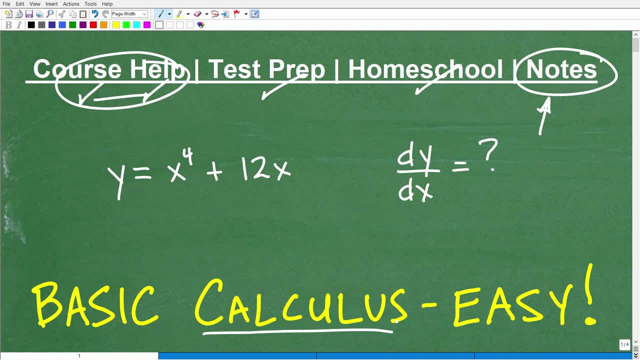 So many problems you know can only be solved with calculus. So kind of reach a point in your high school level, mathematics or whatever you know generally in high school- although some students could take calculus in high school- you reach a kind of point where you can only do so much with 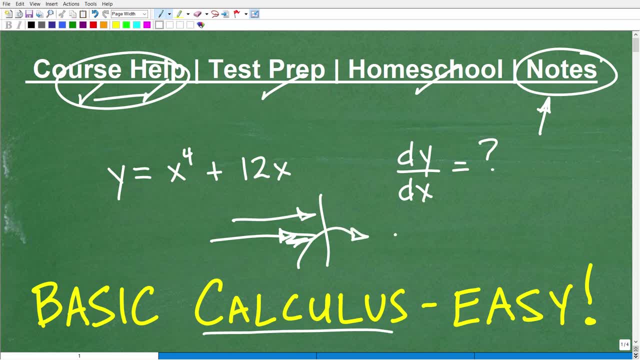 With algebra, you're going to have to jump into this universe of calculus to solve all kinds of cool problems- Very, very interesting mathematics. So I definitely encourage you to to work towards that if you're interested. Now, if you want to know more about calculus, kind of like at a basic level, certainly you might want to check out my videos and my other my other calculus videos in my calculus playlist on my YouTube channel.